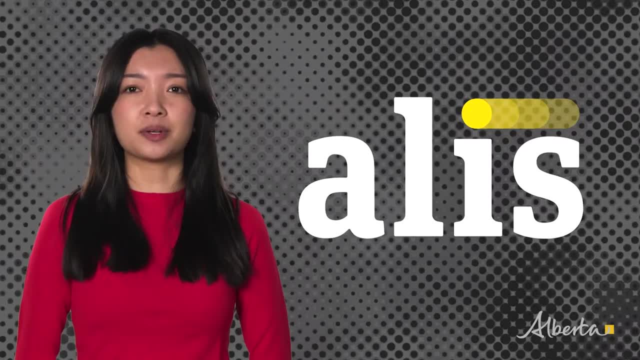 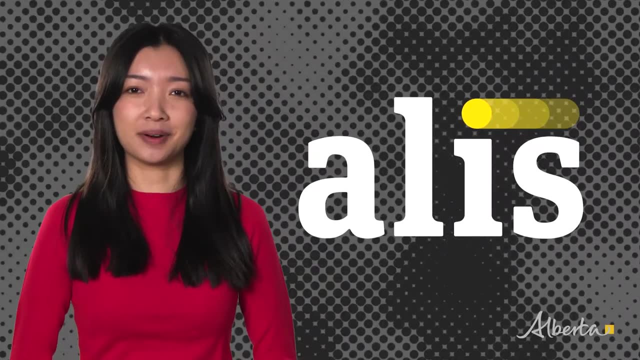 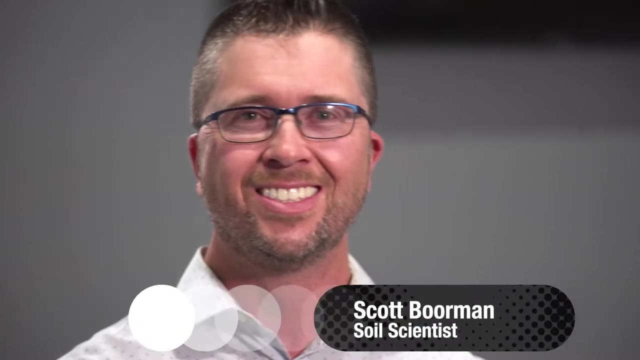 forestry and other industries and for protecting water resources and the environment. To help us get the lay of the land on this earthy career, we talked to a soil scientist working here in Alberta. Hi, my name is Scott and I'm a soil scientist. As a soil scientist, we look at physical and 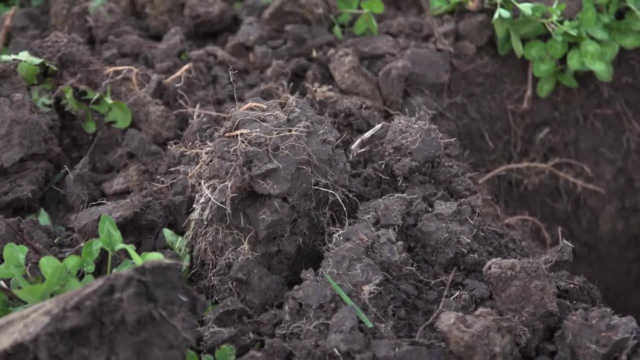 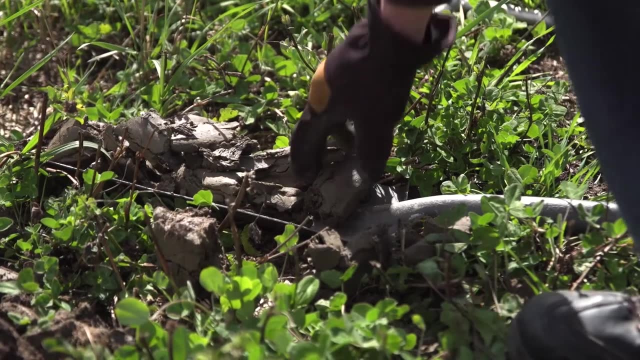 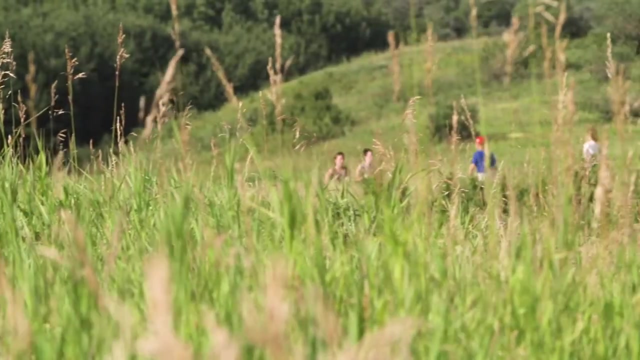 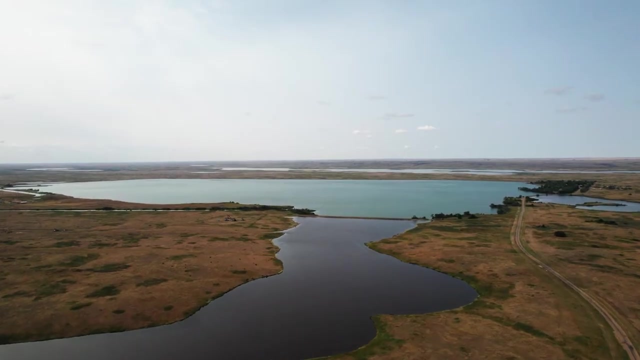 chemical properties to provide information for agricultural resources, environmental studies and water conservation. We look at the interaction of soils with organisms, plants and the atmosphere, and we study the positive and negative effects of human activity on soil quality. The work that soil scientists complete is important to conserve soils in Alberta and to provide the best 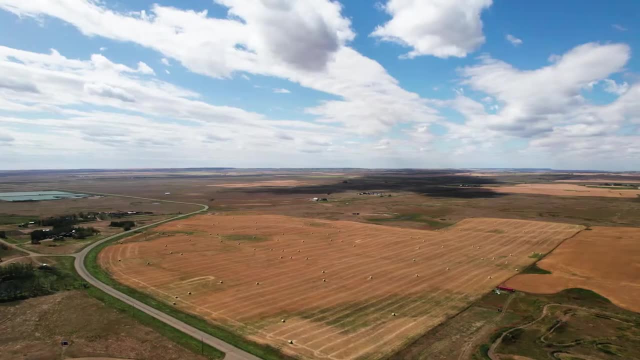 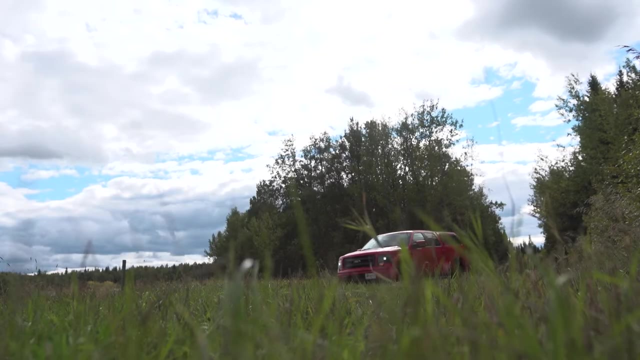 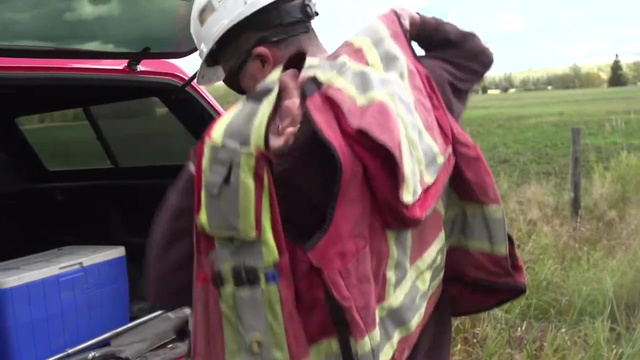 decisions for future reclamation and restoration of ecosystems and natural landscapes. As a soil scientist, you can work in many locations. You can work in private consulting, you can work for the government, you can work with industries and provide various forms of information on that. 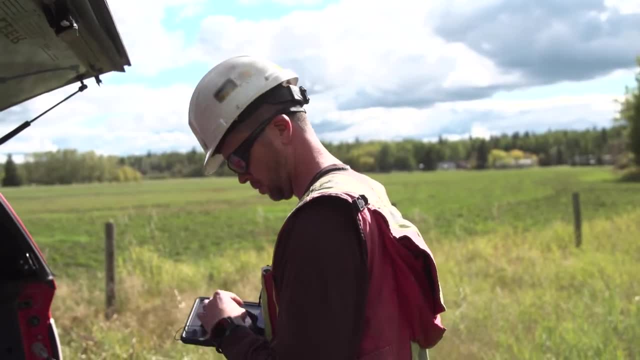 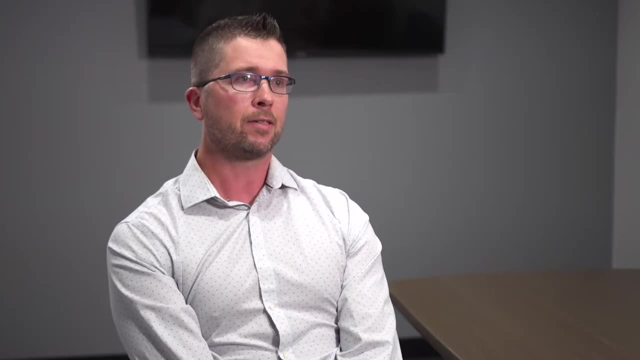 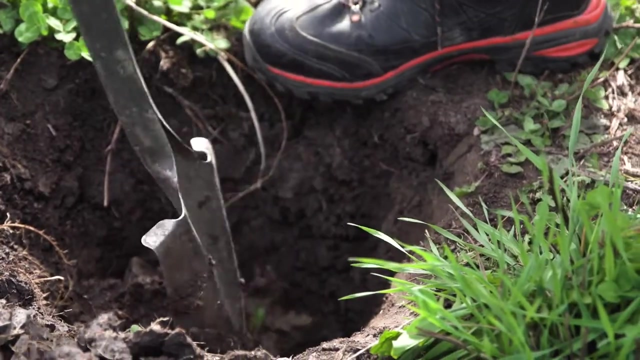 level. Personally, I work for an independent consulting company that deals with independent consulting environmental management and soil issues for oil and gas, agriculture and mining industries. The duties for a soil scientist are highly variable. I complete both fieldwork and office work. When I'm in the field, I collect the data We are digging, soil samples we're collecting. 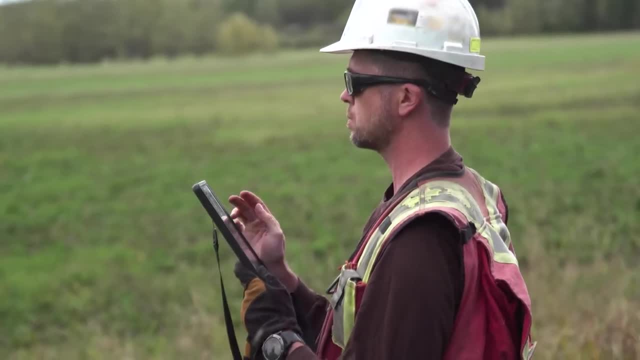 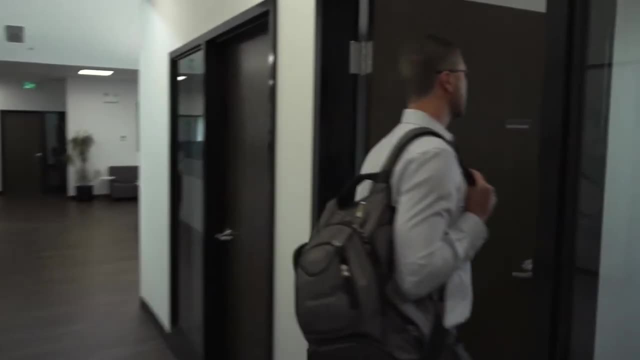 samples to send to the labs. we're mapping the soils in the field and completing the data transition for the client. A typical day for me in the office involves working on reports, coordinating field crews, planning projects and writing proposals for additional work. 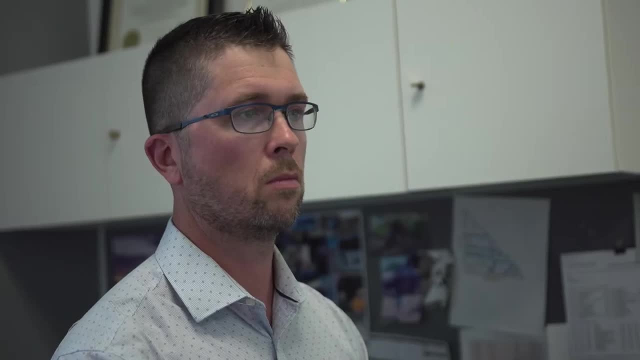 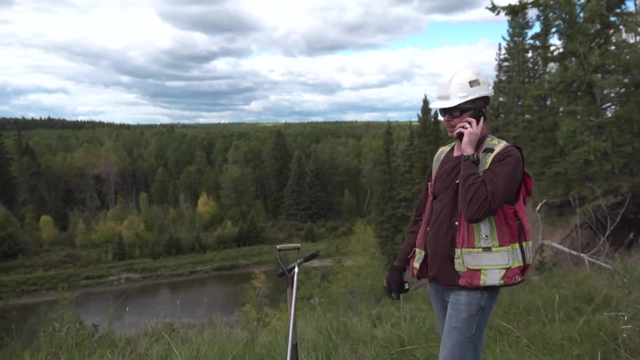 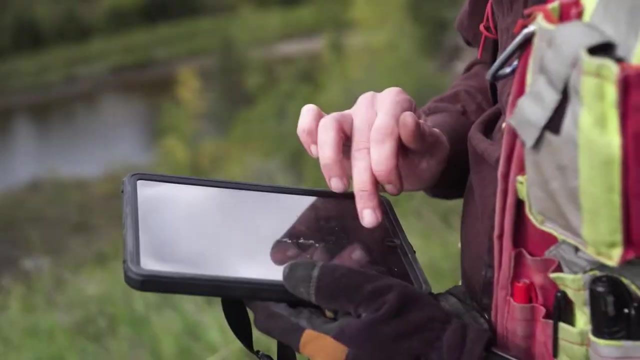 I work with landowners to develop land recommendations for environmental preservation. We survey land by completing soil digs. We evaluate the soil to determine if it's going to be used for reclamation or how the companies can best work with that for reclamation. and 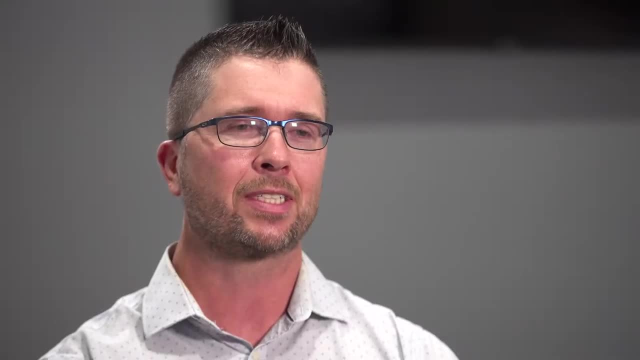 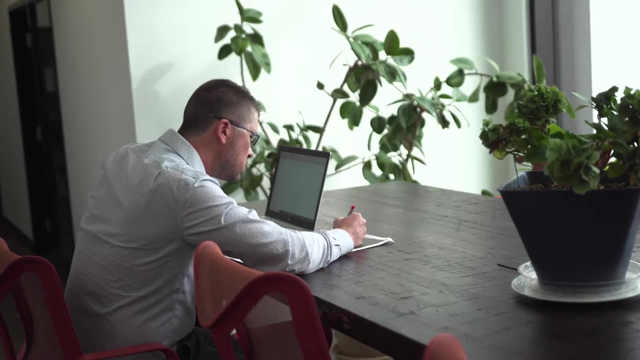 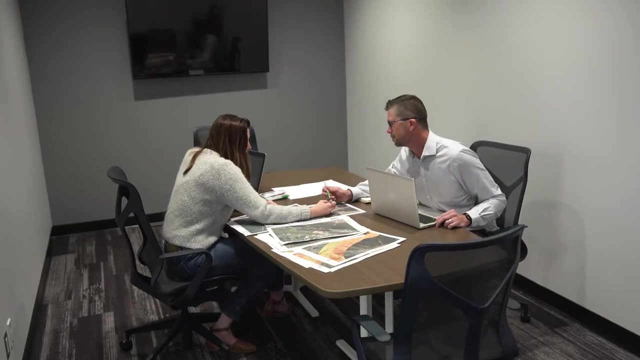 restoration. As a soil scientist, problem-solving skills are very important because the position is and changes on a day-to-day basis with client requests, the weather and field conditions. many things are causing people to adapt. Some other skills you need are the ability to be flexible and communication with your team and clients. 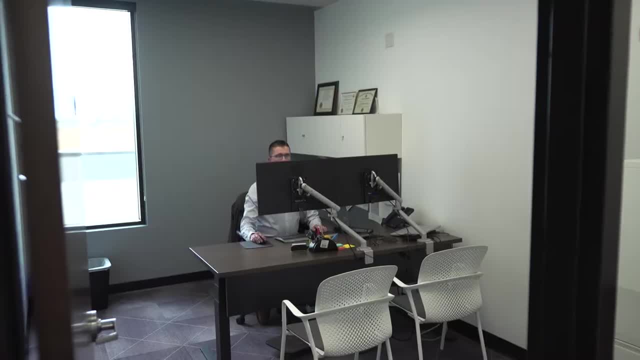 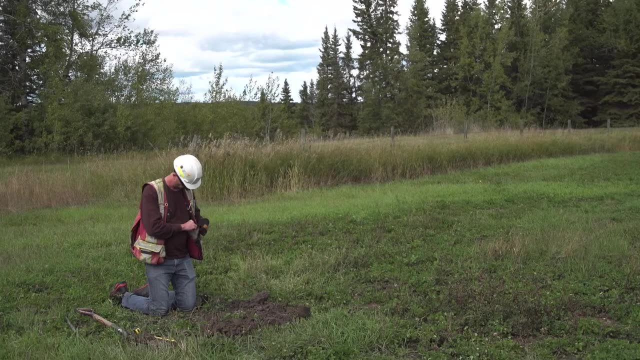 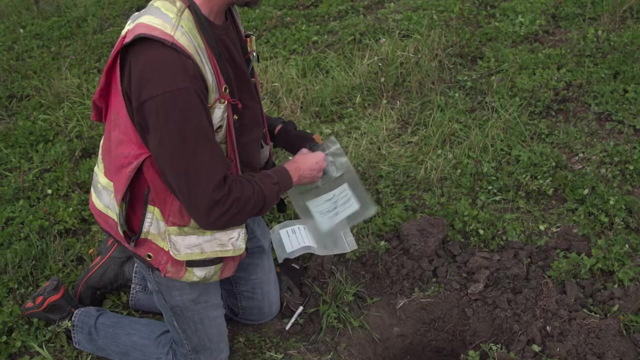 is also an important skill to have As a soil scientist. writing skills are very important for communication to clients and landowners, and also the desire to be outside. Our hours are highly variable. During the busy summer seasons, we are working in the field for extended periods of time. During the winter, we're 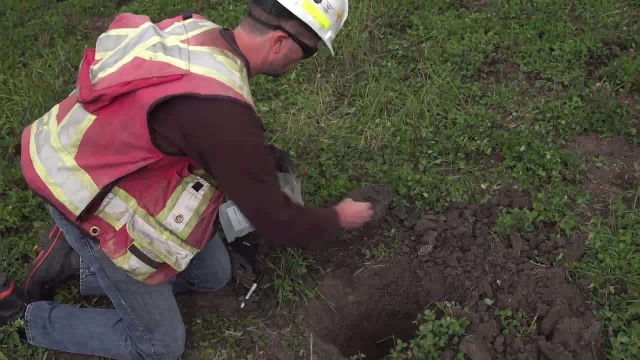 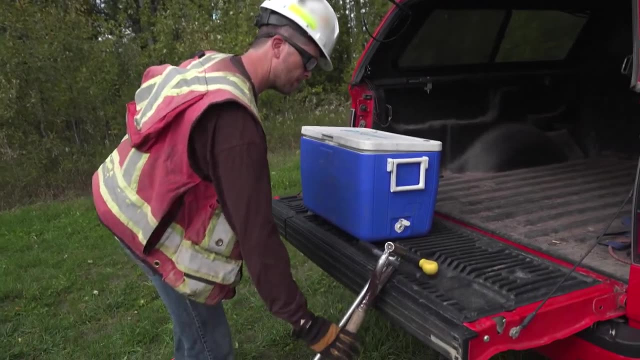 typically in the office working on reports and compiling data for clients. For most of the work we do as soil scientists, travel is a big part of the job. We travel throughout Alberta and throughout Canada for some of the projects that we're involved in. 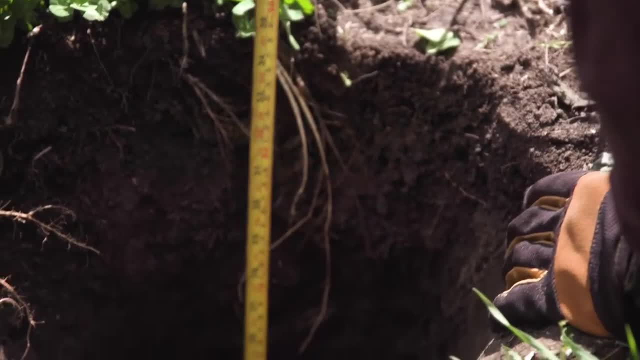 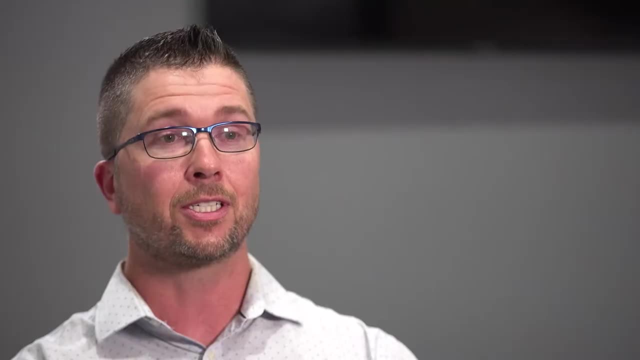 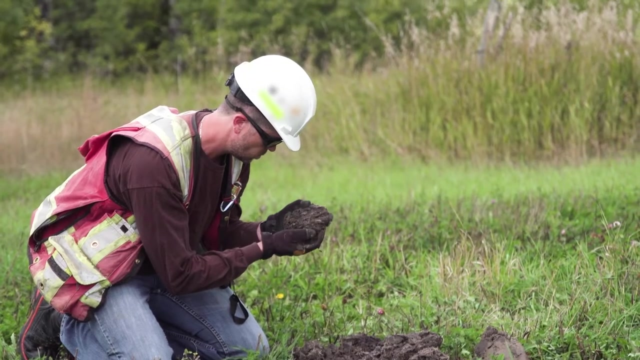 The minimum education requirement for a soil scientist is a Bachelor of Science. This could either be in agricultural, biological or forestry, earth or environmental sciences. It should include a specialization in soil science If you want to continue and specialize a master's or a PhD in applicable fields. 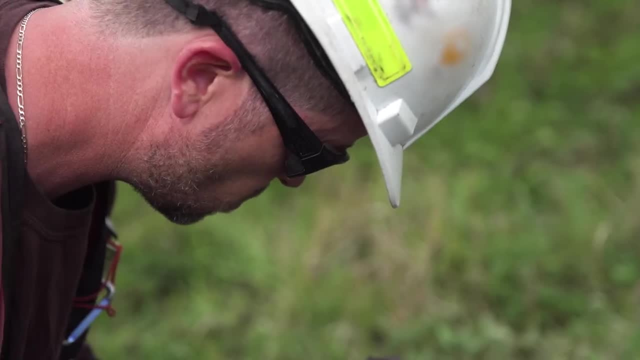 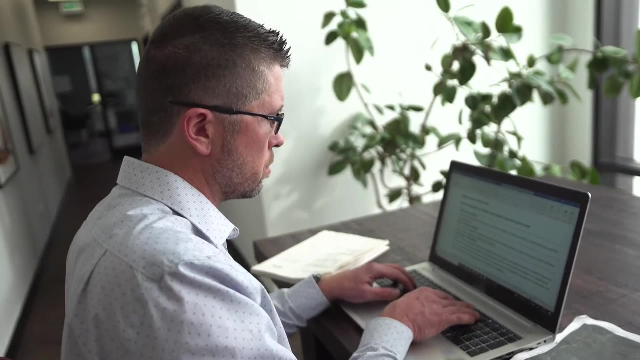 would also be helpful As a soil scientist. you can advance in your career by becoming a project manager, a long-term planner. you can become a research specialist. you can become a research specialist. you can become a specialist. There are many possibilities for advancement in your career. I would 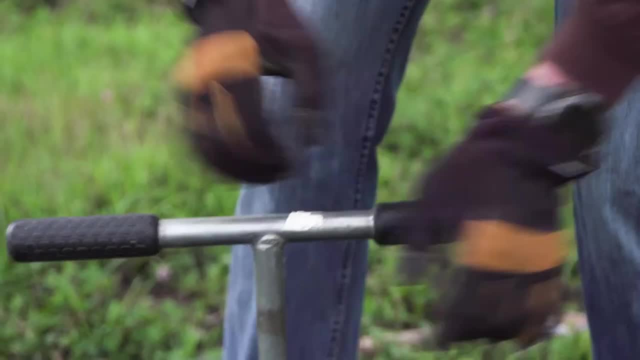 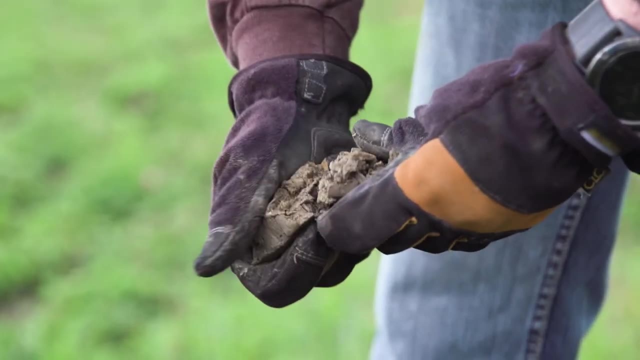 recommend a career as a soil scientist because it's highly dynamic and it allows you to experience a lot of areas and places that most people don't get to see. You get to work outside and you also get to be part of a team in every setting. One of the things I'm most proud of as a soil scientist is working on 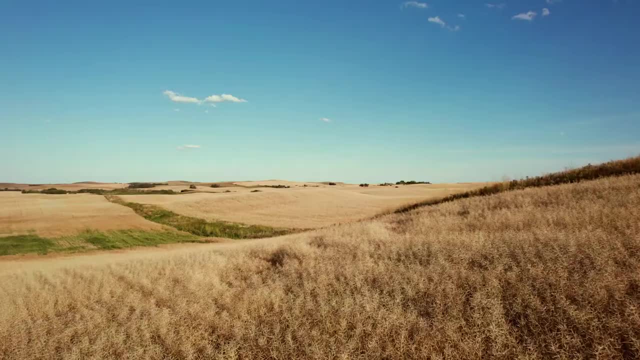 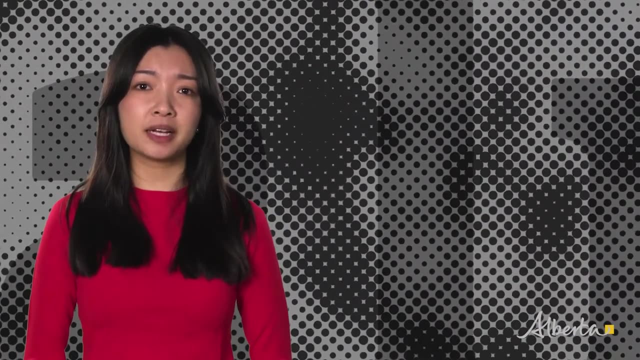 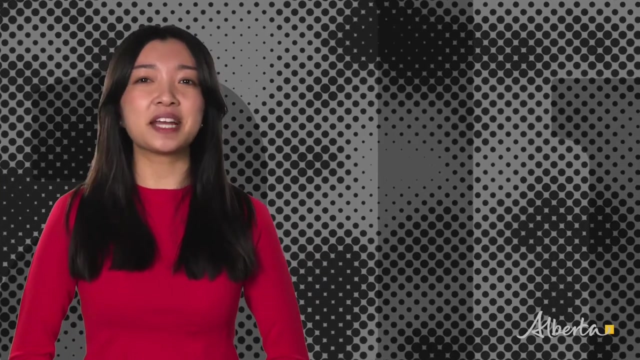 projects and being involved to see landscapes being reclaimed and restored to their original states. This career needs a good ability to communicate with the public, members of industry and government. It also requires health and stamina to work outside in various locations. If this feels like your turf, you'll be outstanding in your field As a soil. 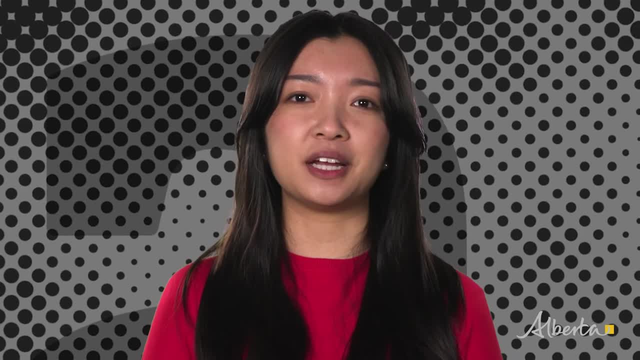 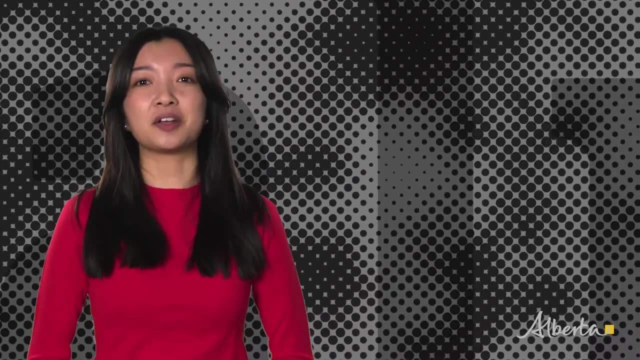 scientist. dig around for more information about this occupation, including training requirements and salary ranges, in the occupational profile on the ALIS website. While you're there, check out related occupations such as agrologist. Explore the possibilities. Go to alisalbertaca. For more information, visit alisalbertaca.